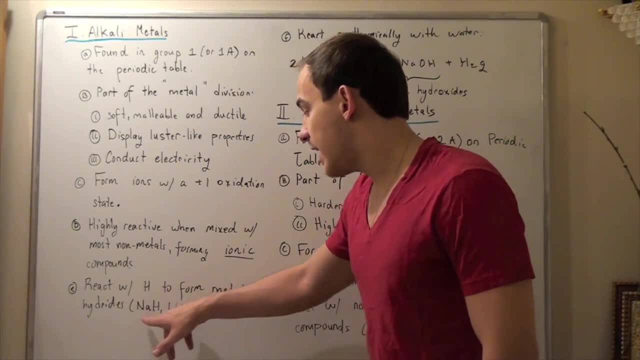 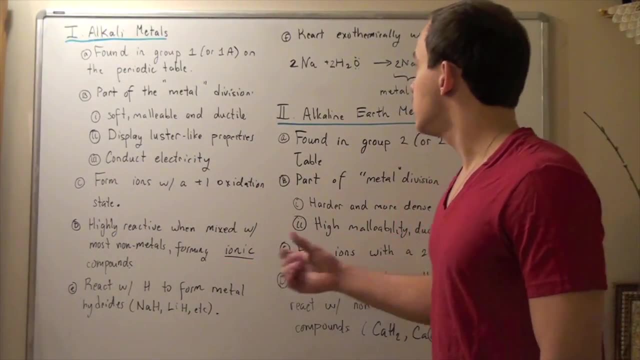 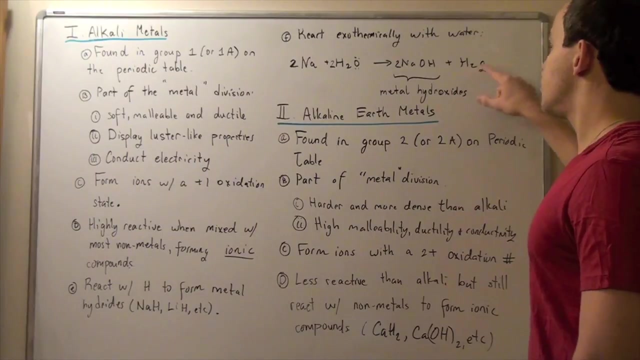 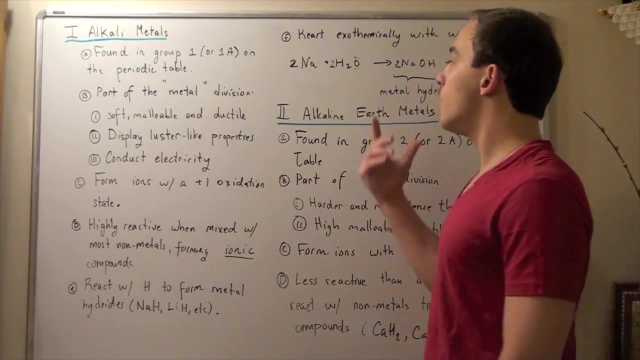 LiH, etc. in which the Na and the Li both have a positive one oxidation state. Now if you mix the metals with water, they will react exothermically to produce a metal hydroxide and that is called a H2 gas. So, for example, if you mix two moles of sodium in a solid 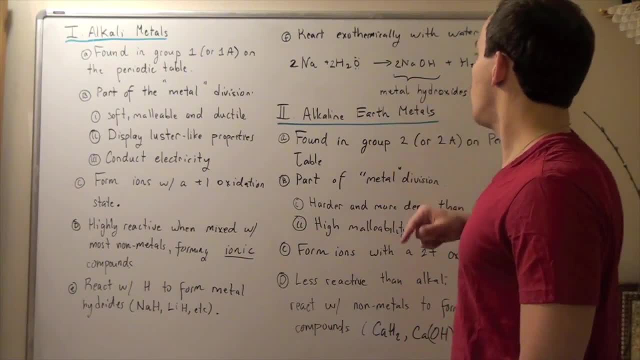 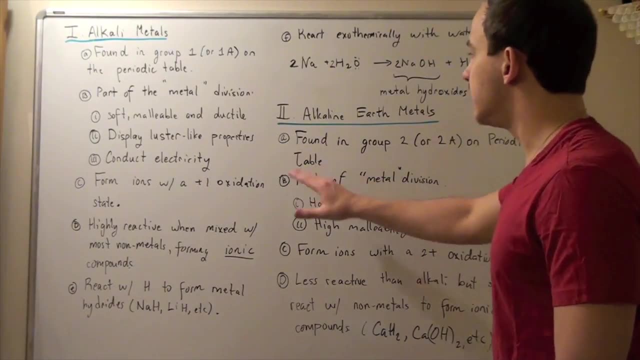 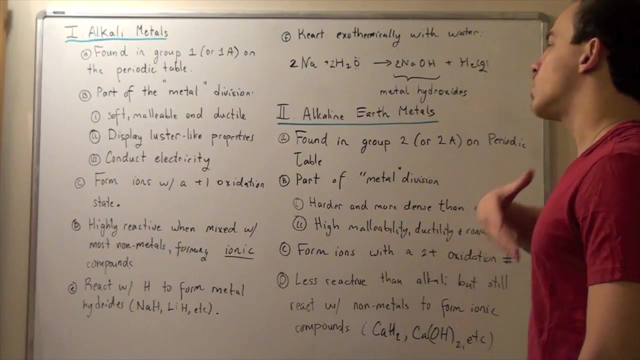 state: with two moles of water, you'll get two moles of metal hydroxide and one mole of H2 or diatomic gas. Now let's look at the second type of group, right next to our alkaline metals, known as alkaline earth metals. Now, these guys are obviously in group two or group 2A on the 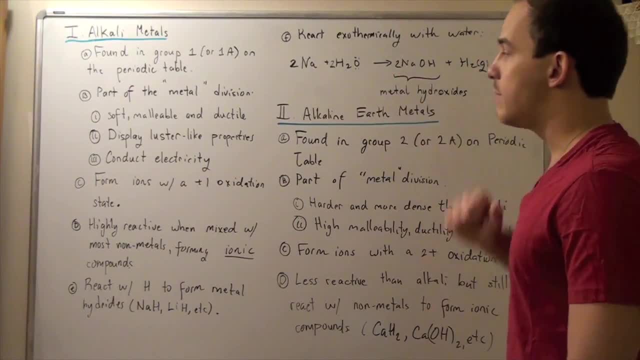 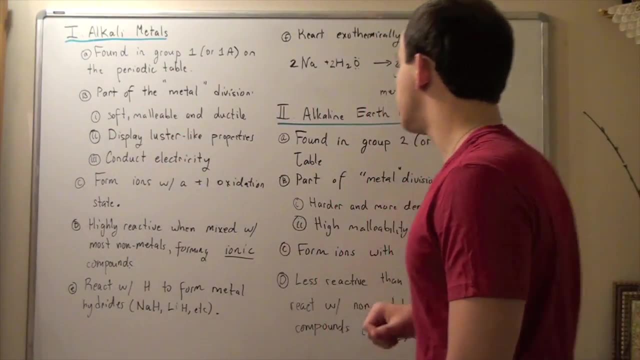 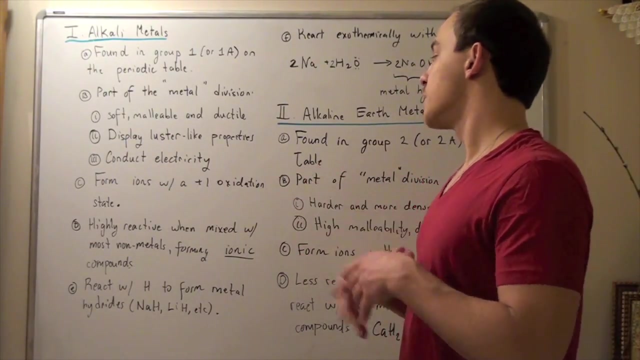 periodic table. and these guys, just like the alkaline metals, are also part of the metal division. so they're metals. but unlike these guys, which are soft, these guys are harder and more dense. that means their molecules in a solid state are closer together per unit volume. now, since they're metal, metals they're also. 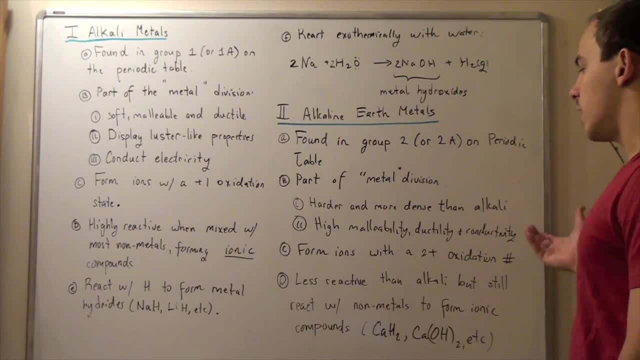 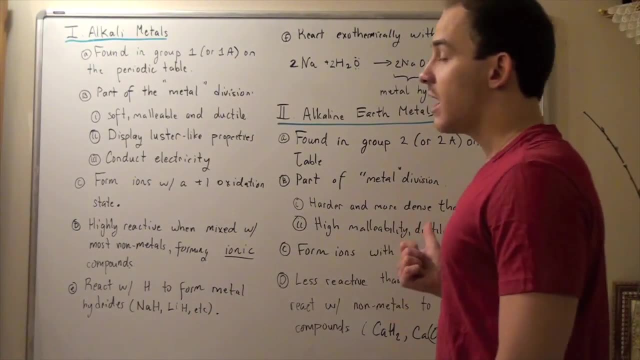 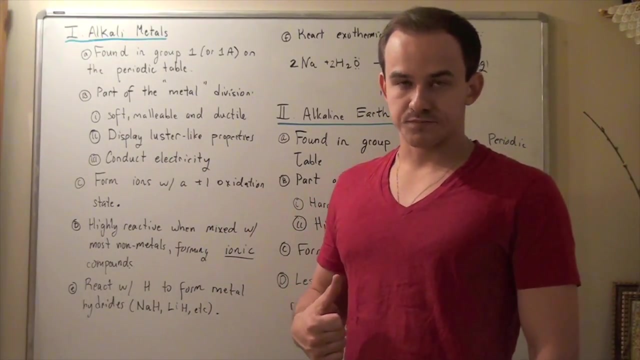 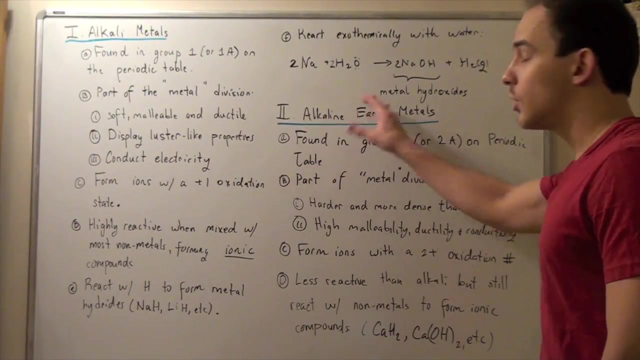 malleable, ductile and they conduct electricity well. now these guys, unlike these guys, form plus two oxidation state. in other words, these guys lose not one electron but two electrons when they react with our nonmetals. so that means they're more likely to lose electrons now. our alkaline earth metals are less. 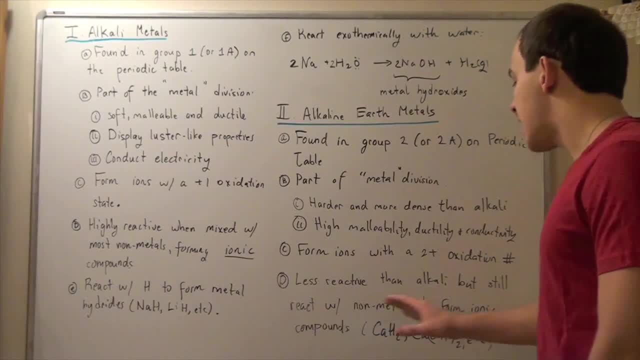 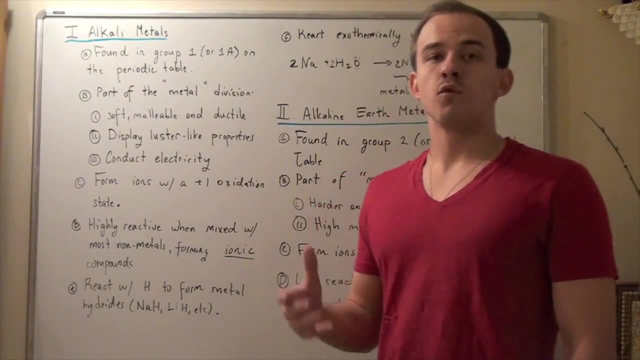 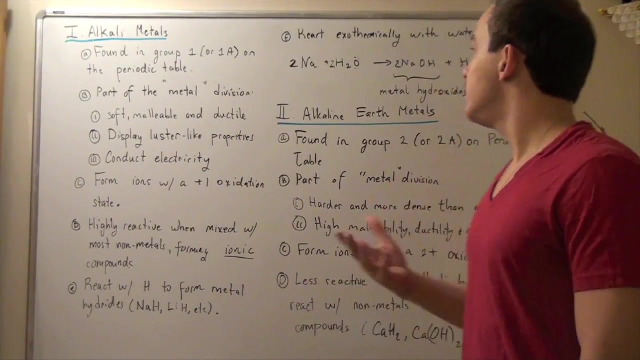 reactive than the alkali metals but still react with the nonmetals to form ionic compounds. for example, calcium reacts with hydrogen and sodium, and calcium reacts with hydrogen and sodium and calcium to form calcium hydride, CAH2, and calcium also reacts with hydroxide when. 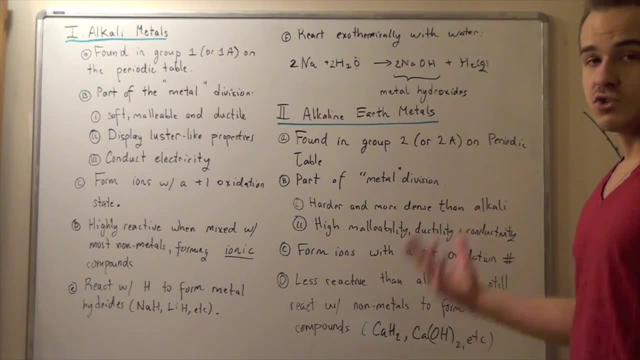 we mix them with water to form our calcium hydroxide molecule, in which we have two hydroxides, because each hydroxide has an oxidation state of negative one. so to balance out the plus two oxidation state on our alkaline earth metal, the calcium, we need two of these guys. 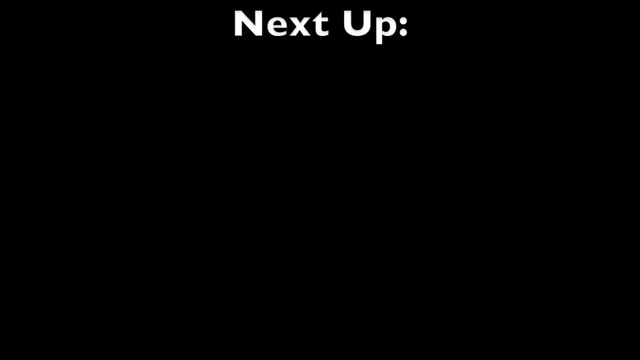 here in this graph you can see the same thing we've already seen in the graph, but we've already seen these three different levels. here in the graph you would see these two alpha and beta and these two hydrogen and sodium hydride units are similar, but you notice the differences in chemistry between these.